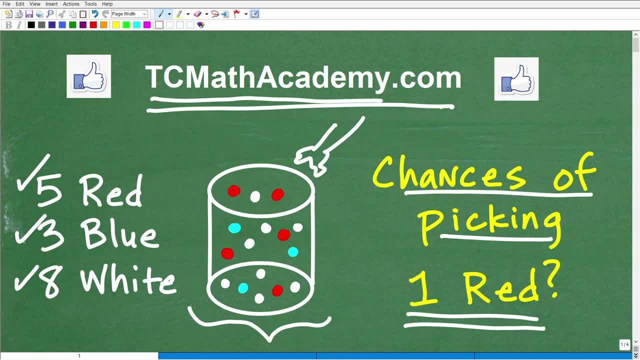 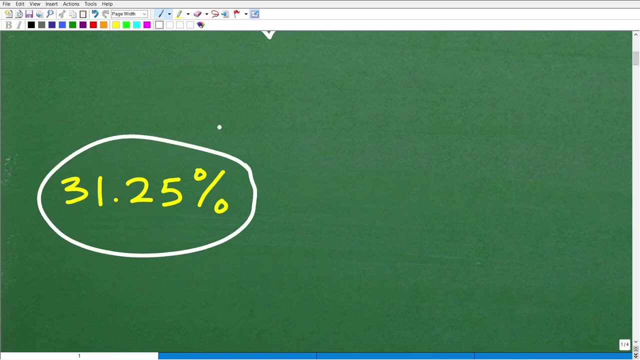 tcmathacademycom. You can find a link to it in the description, And if this video helps you out, don't forget to like and subscribe, as that definitely helps me out. Okay, so let's go ahead and take a look at the answer. The answer is 31.25%. Okay, so again. 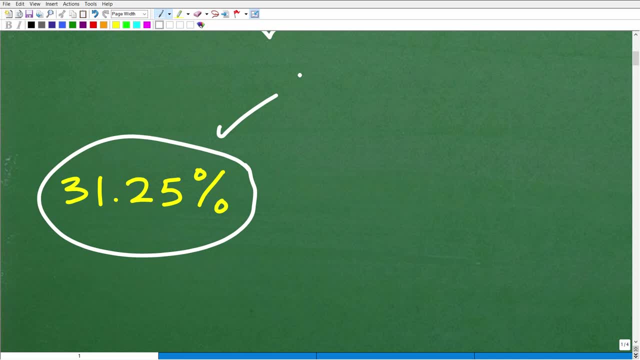 we're talking about basic probability and even if you forgot about probability, you probably reasoned through logically and figured this thing out. I don't think it's too difficult, Again, even if you know the math involved. but you know, I think common sense, you know, would probably allow most. 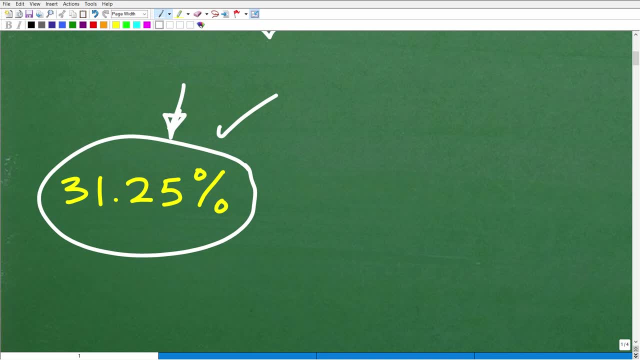 people to arrive to this particular answer. But anyways, if you got this right and you knew exactly what you were doing, let's go ahead and give you a nice little happy face in A+, a 100% and a few stars, so you can tell your friends and family that you know a thing or two about basic probability. 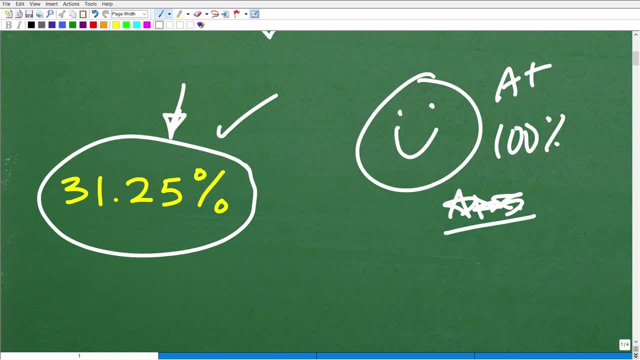 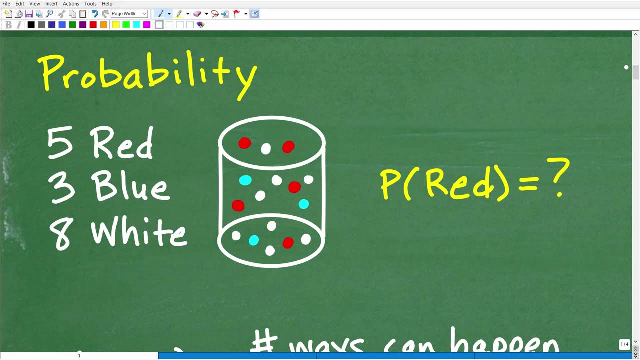 They'll be very impressed with that knowledge. Okay, so let's go ahead and get into this right now. Again, we are talking about probability, So the original question is: what are the chances of something happening? Anytime we're asking questions like: hey, what's the chances? 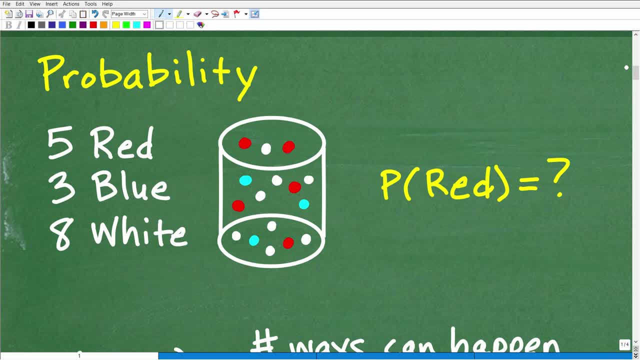 of rain this afternoon, right? Well, another word that's synonymous- you know that we can exchange for the word chances- is probability. What's the probability of rain, What's the chances of it raining That type of thing? So we're dealing with probability. Now probability. 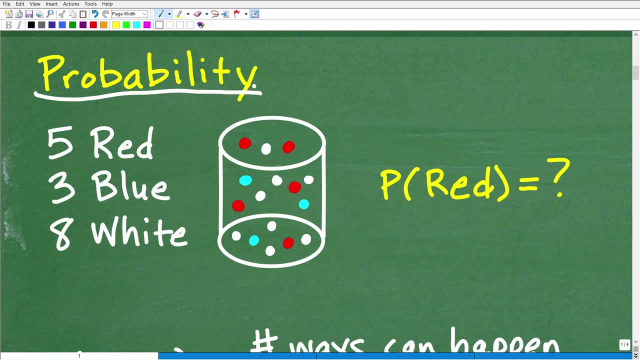 is a type of mathematics. okay, And what are we trying to do here? Well, we're trying to make predictions And you know, probably it's a big, big topic in math. So you should know at least some real basic concepts about probability. The first is: probability is: 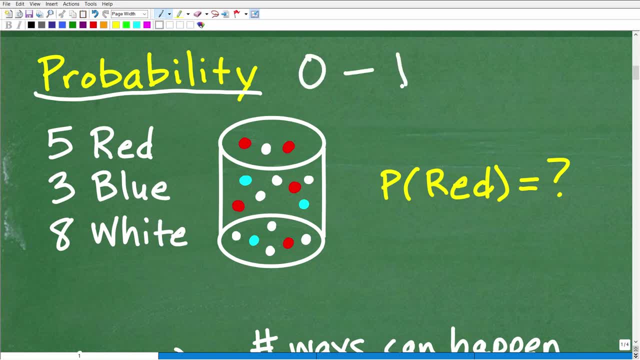 measured between zero and one, technically speaking, But really we measure things. We like to express probability in percent, So anywhere from 0% to 100%. So let's go back to our question about rain. What is the chances of rain this afternoon? Zero percent, right, Or? 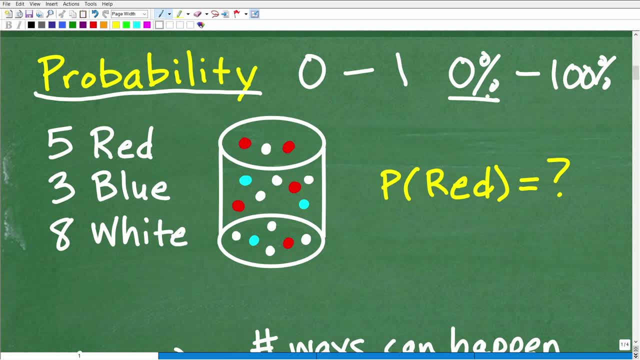 100%. So if you said zero percent, it's absolutely not going to happen. If you said 100%, it's 100%, guaranteed it's going to happen. And, of course, everything else between just gives us some sort of prediction on. you know the odds, the chances of something occurring. Okay, so there's a lot to know. 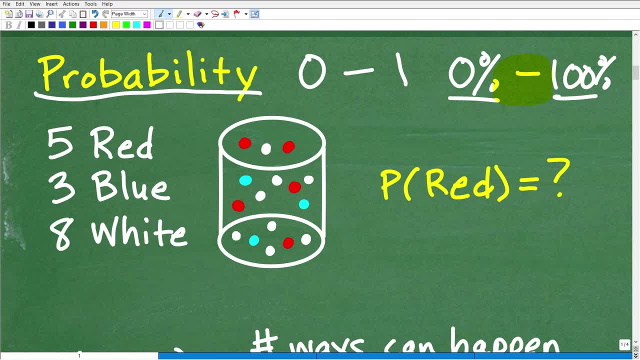 about probability, But this particular problem is a very, very basic introduction to probability. Okay, so, with that being said, let's go back to our question. So what are the chances of rain? this afternoon, We did a math test, you know, ok, so what happens if you select a characteristic? 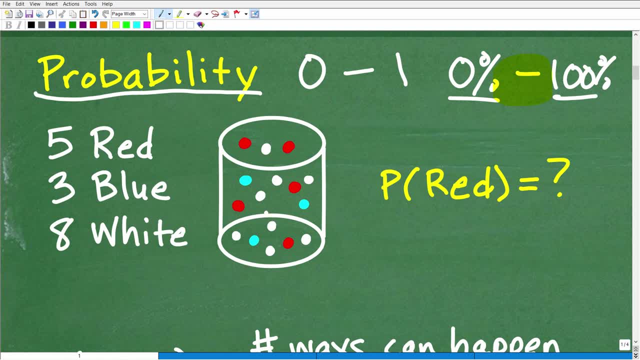 Sure, Robertany Red. Why is that? the probability, The probability of rain is the 놀� he can find is always the probability of rain, right at the prince of the ring. the correct answer So in this case, Robertany Red, is the probability of rain. 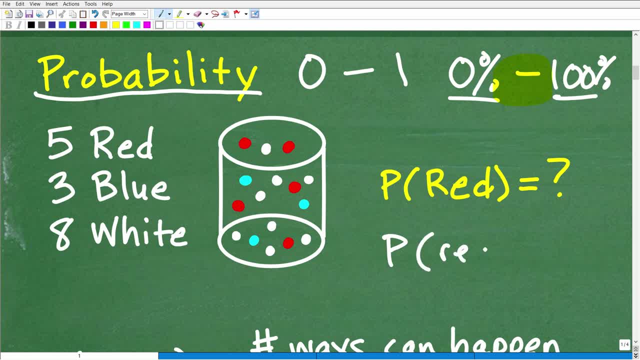 So, instead of the probability of rain, what we can do is find the probability of a red on our lab stage. So for theMSB, we wanted to do is find the probability of red, of us selecting one red, and one way we can write that in terms of notation, mathematical notation is this we can: 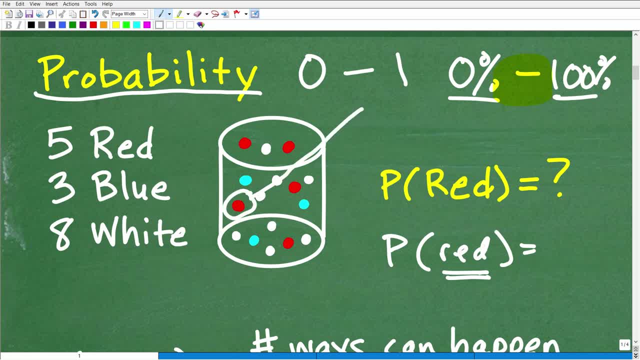 work with Bern. you see here Janet Palin. second, this is below machines. they olsa by the personell of a physical microorganism local To avoid that red marble. or maybe we grabbed this red marble or this one right, but of course we put our hands. 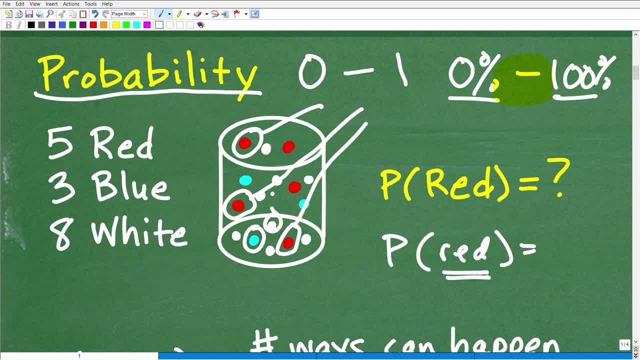 into the jar and we're just grabbing one marble. we could grab a blue, we can grab a white. there's other things that could happen, right, but specifically, what's the probability of red? well, we're going to have to want to know the basic definition of probability. okay, so this is a nice 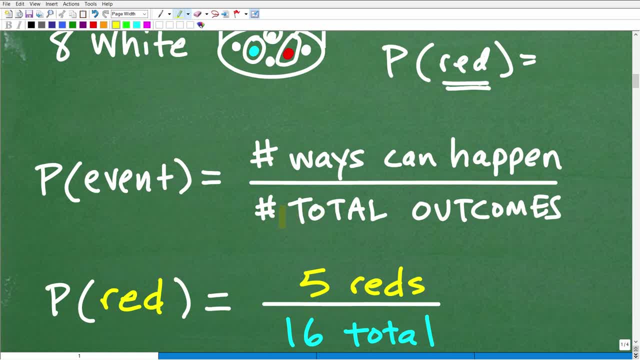 kind of easy to understand, hopefully a way of defining probability. now there's more formal ways to define it, but effectively they say the same thing. so the probability of an event occurring okay is the number of ways that event could happen okay, over over that or divided by the. 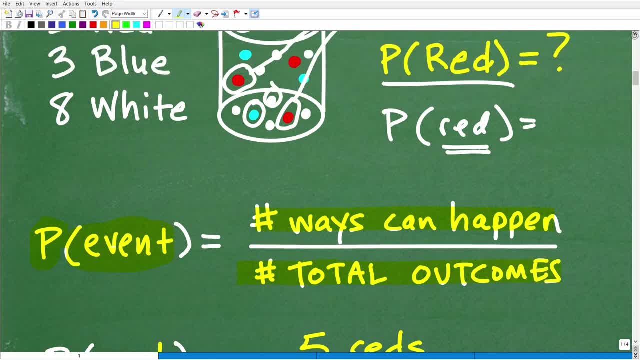 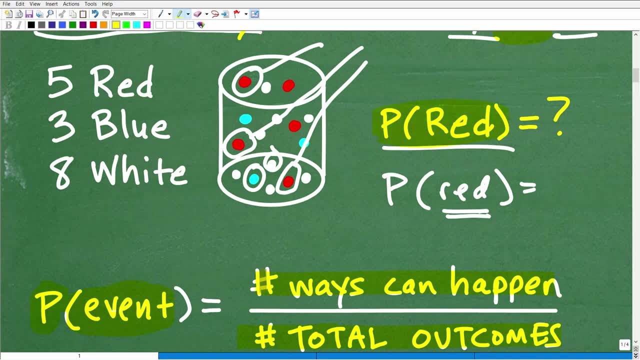 total number of outcomes. so let's go back to our jar here. right? so you're going to stick your hand, you're going to grab one marble. so how many different ways could you get a red marble? well, we got one way we can get this red. right, you could have grabbed this red or that one there. that's one, two, there's three, there's four. 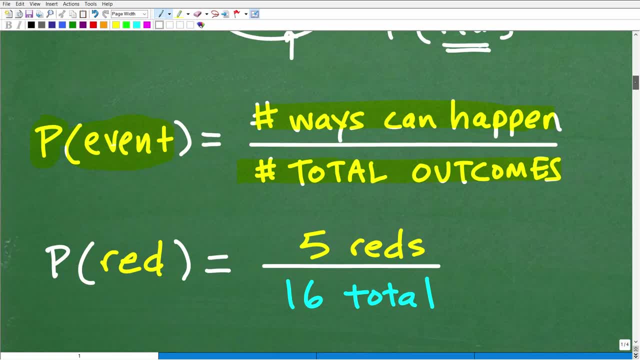 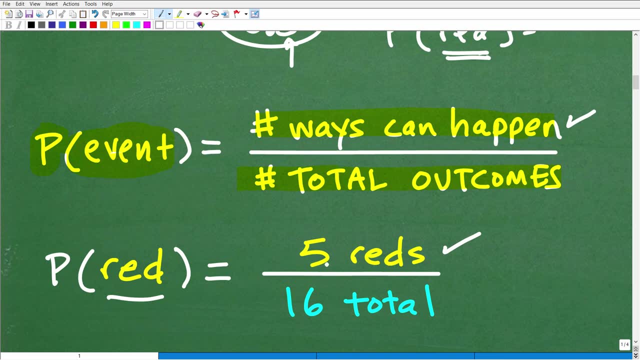 there's five. so you know, grabbing a red marble could have happened in five different ways, right? so the number of ways, the probability of red occurring, well, there's five ways, right, because it's five marbles, uh, individual marbles you could have grabbed, but what's the total number of? 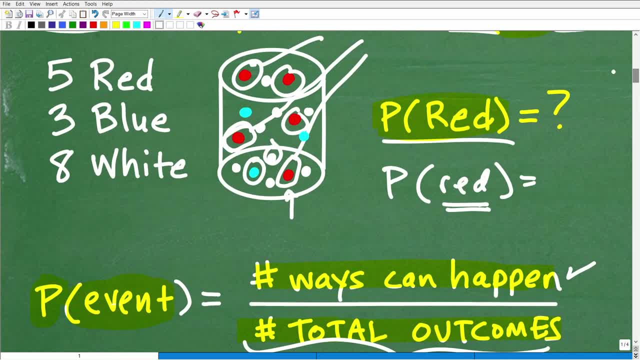 outcomes. well, how many marbles could have happened in five different ways? right? so the probability in total do we have? Well, 5 and 3 is 8 plus 8, and 8 and 8 is 16.. Okay, there's 16 total marbles in. 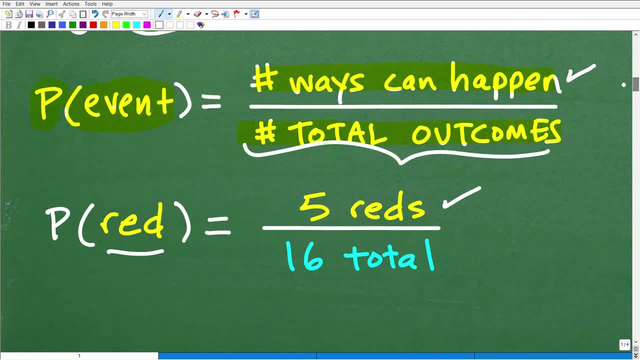 here. So that's the total number of outcomes. all right, So we have 5 reds over 16. total right, So here we have a fraction: 5 over 16.. But again, most of us are familiar with probability in terms of. 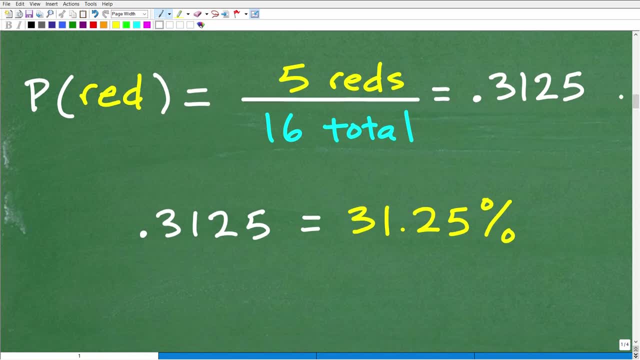 it being expressed in terms of a percent. Okay, so how do we change 5 into 16, into a percent? Well, just take 5 divided by 16.. We get the decimal 0.3125, right, So you know, this would be the. 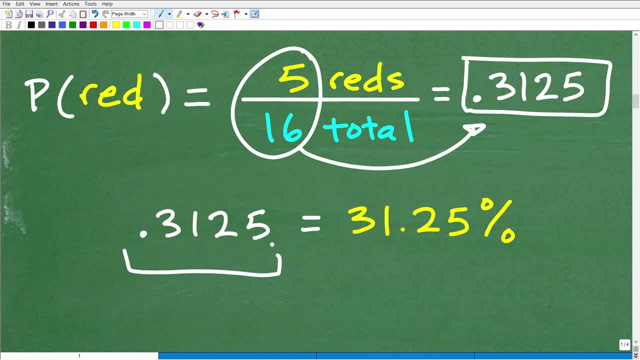 correct version of the answer. okay, Let's just say this much: If you answered 5 over 16- or 0.3125, I also would have to give you a nice little happy face. But for those of you that took it, 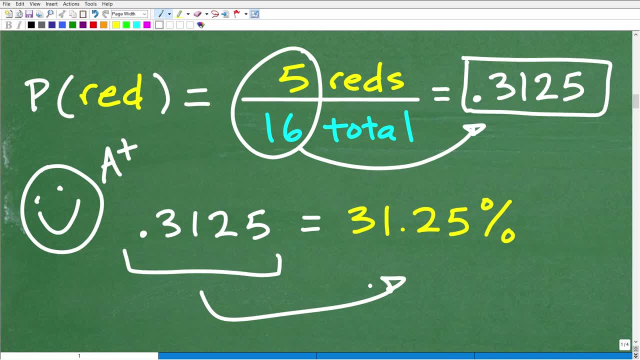 to the next level, I would have to give you a nice little happy face. But for those of you that took it to the next level, I would have to give you a nice little happy face. But for those of you that took it to the next level and gave me this as a percent, you get an A plus. all right. 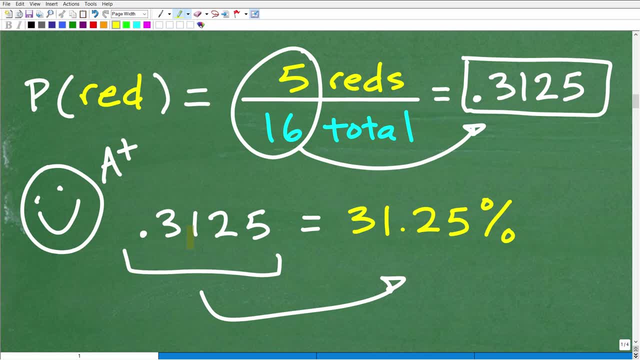 There's nothing wrong with these answers, But again, we're more used to seeing probability expressed as a percent. So how do I change a decimal to a percent? Well, pretty easy. All we need to do is move that decimal point over two places to the right or multiply by 100. And you. 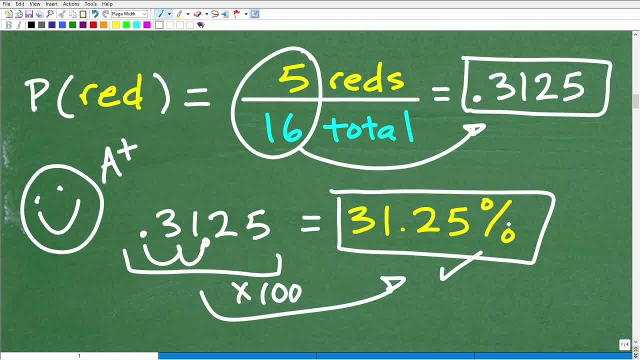 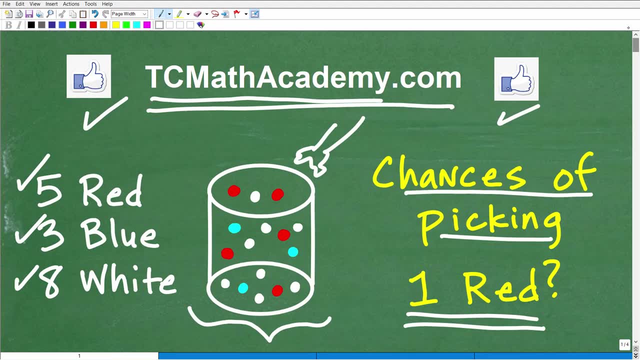 end up with 31.25%. Okay, so probability is a huge topic and a very important topic. You know, if you just, like you know, watch the news, or you know read the newspaper or any information you know, or you know watch sports and whatnot, they're always talking about probability of this. 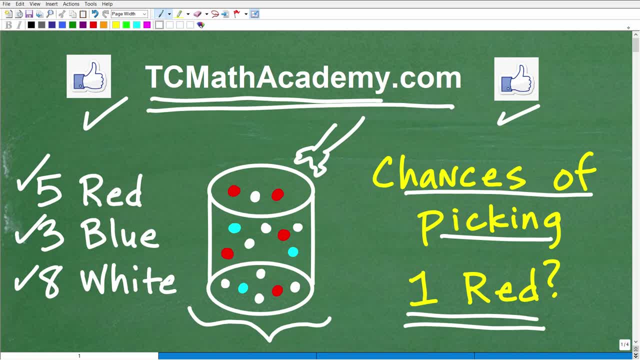 probability of that, even the weather right. So you know, anytime you see probability or the percent symbol, okay, it's a good, you know, it's a good idea to have some idea of what's going on. But if you really want to get into probability and learn it, you're definitely going to have to.